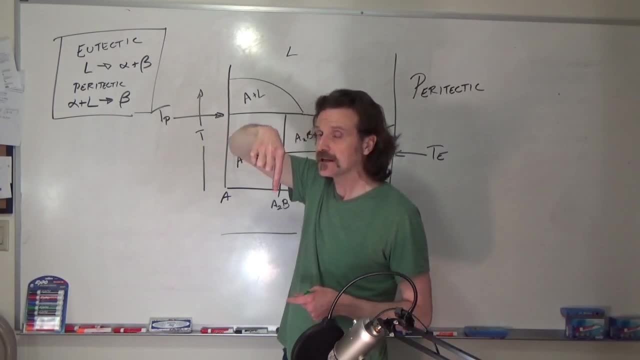 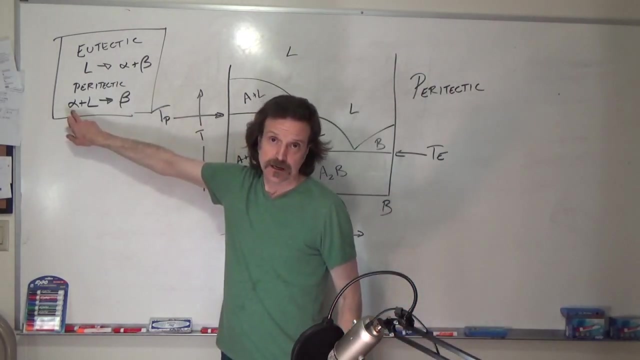 So you're going through the eutectic temperature at the eutectic composition, and the liquid transforms into two solids. In the case of the peritectic, we have two phases, an alpha and a liquid transforming into a single solid. 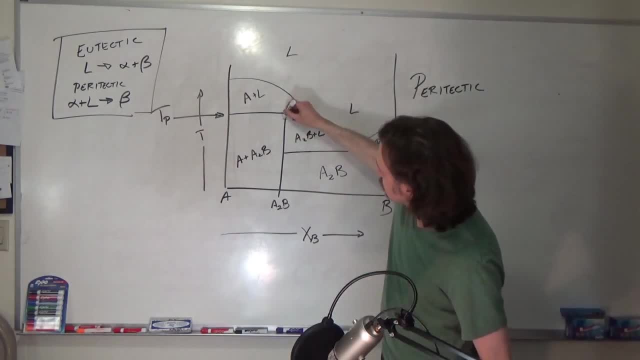 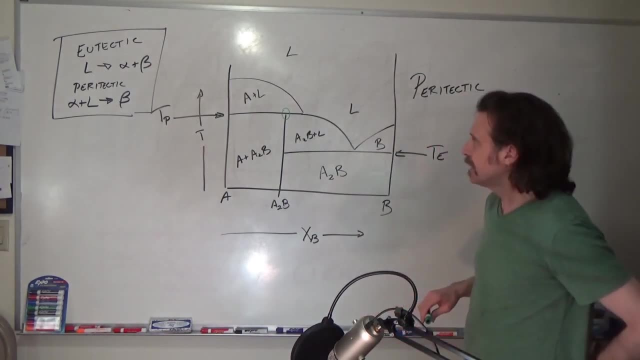 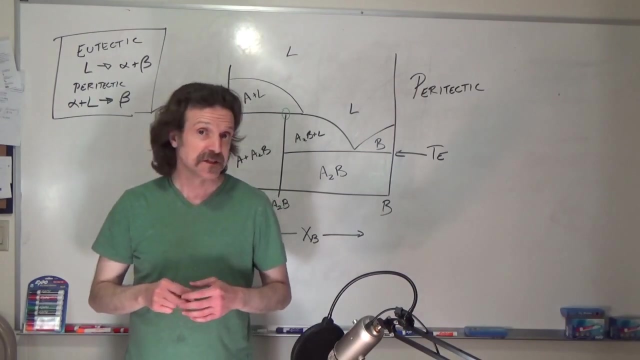 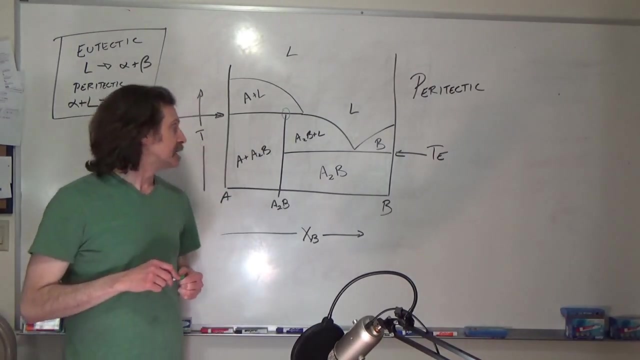 and that is what's happening right here. So I drew these as line compounds because it's a little bit easier to see. The peritectic is very important, particularly in ceramic materials. It is a little bit tricky. 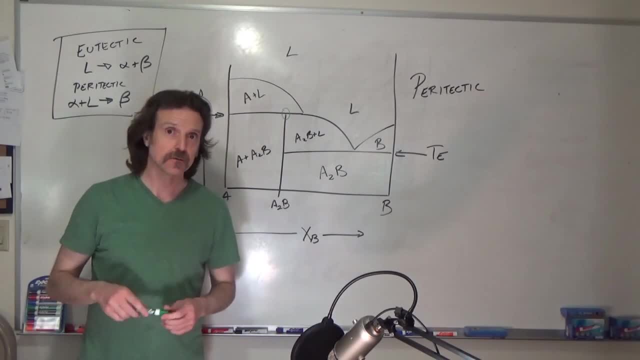 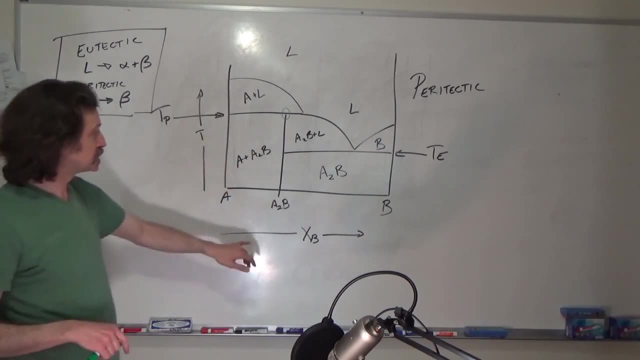 And I'll show you kind of the way to make sure that you get it right. But let's look at this. So what we have is we've got a line compound and we're talking about temperature on the y-axis b or your composition on the x-axis. 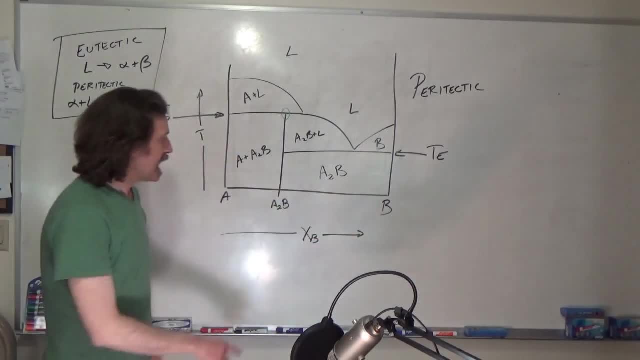 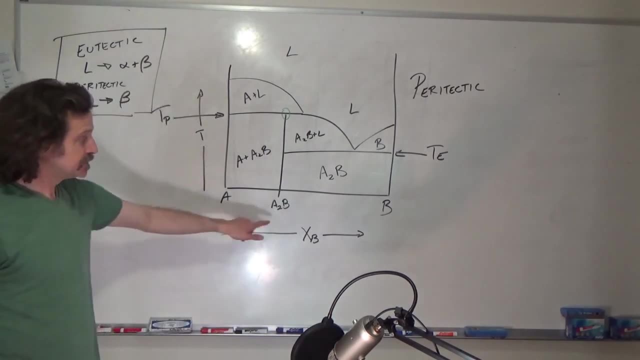 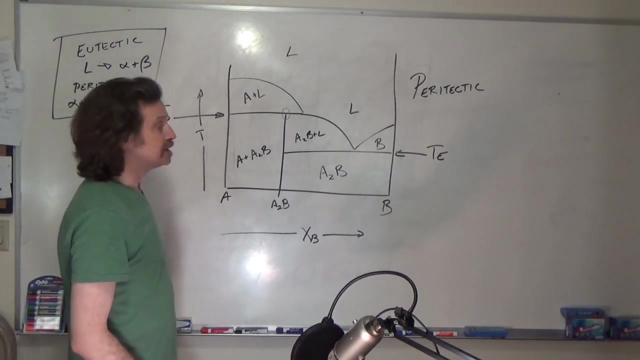 and we have, you know, composition a, b, and then I made a stoichiometric compound between them. So this is a to b, And then I drew in the components in the phase diagram. And again you're looking at this and you say to yourself: 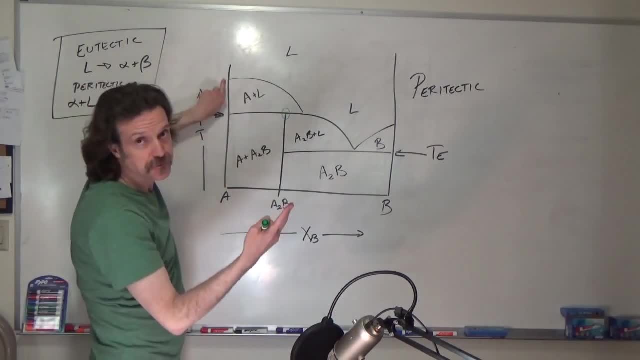 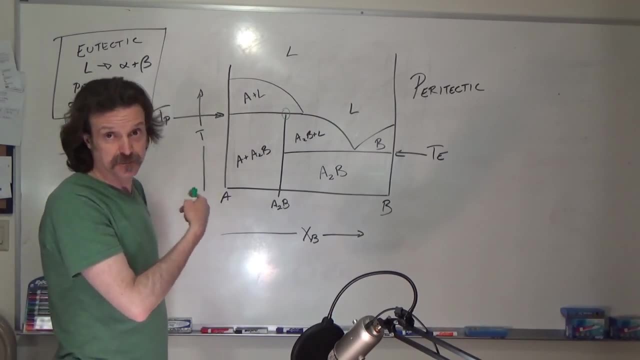 well, okay, I've got a, I've got liquid. therefore, I have to have a two-phase region, And this is something that many phase diagrams that you're going to find in textbooks, and particularly in literature, they don't have the names filled in. 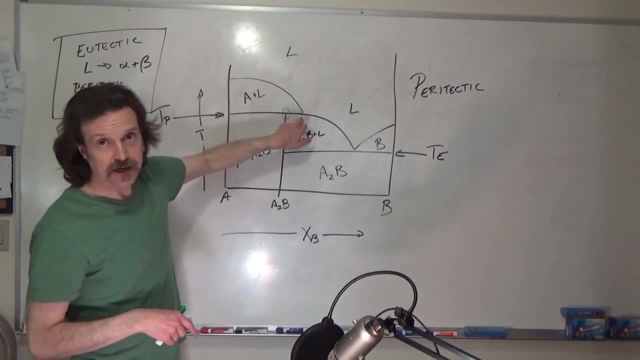 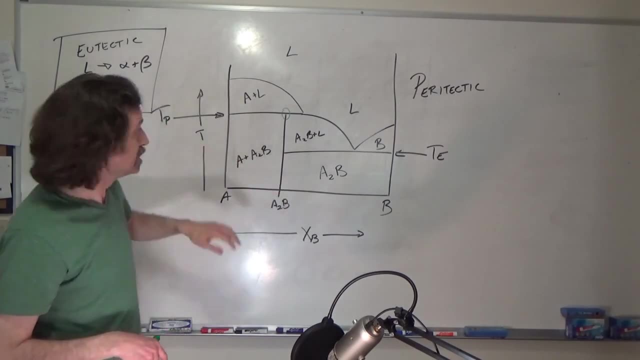 They just give you the lines and they might write the temperatures or the compositions, but they don't leave the naming, and that's something you have to fill in. So that's why I filled it in here for you, And you should probably practice that on your own. 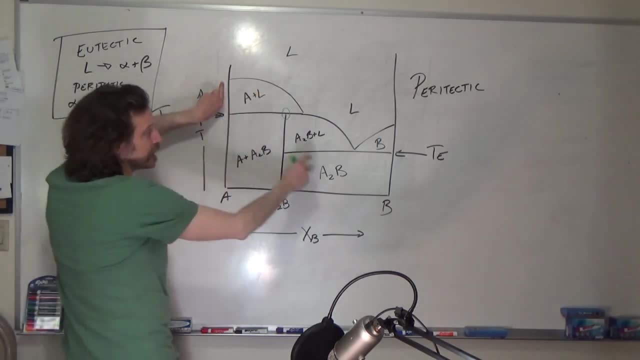 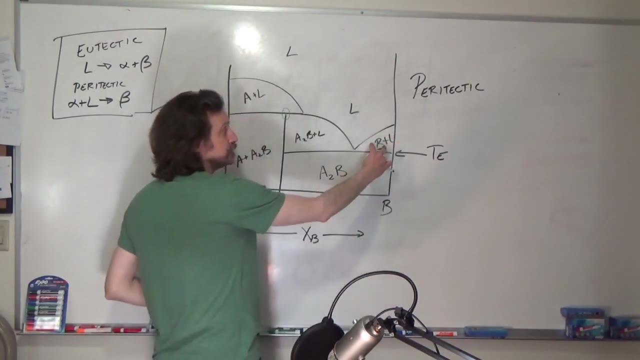 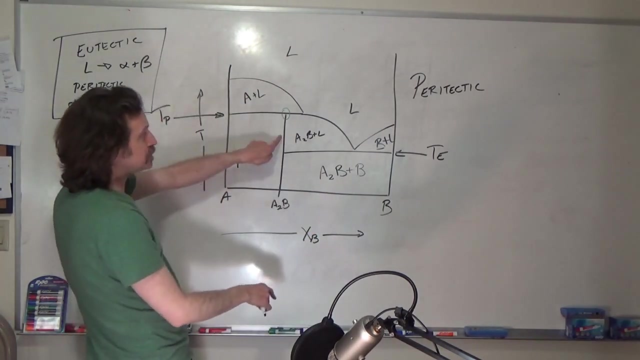 But I've got a liquid two-phase region. I've got B liquid two-phase region. I've got A to be a two-phase region. I've got a to be B Two-phase region Here. I've got a to be liquid Two-phase region and I've got B liquid two-phase region. 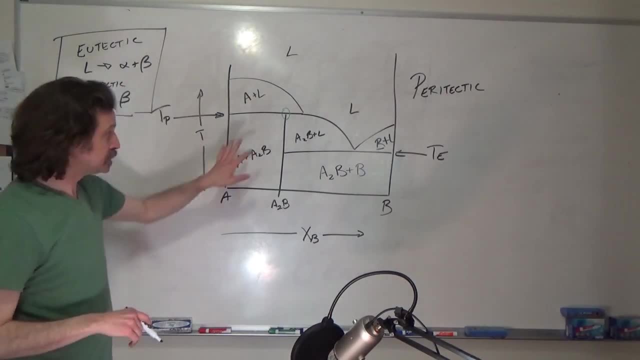 so everywhere that there should be a Two-phase region separating single-phase regions. We have those, So you know whenever you're you're Filling these out. the easiest way to do it is to start on You know one side and work your way across if you get stuck. 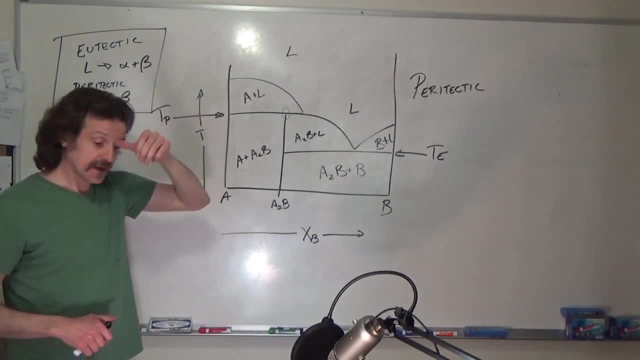 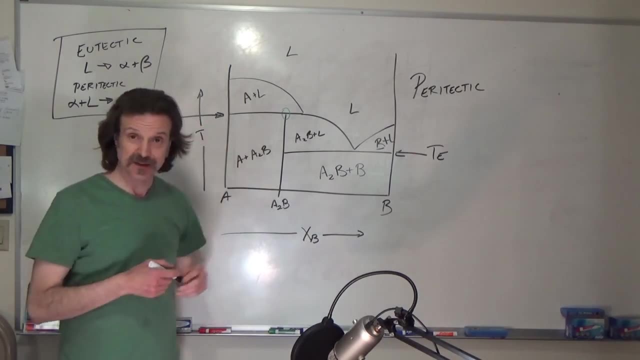 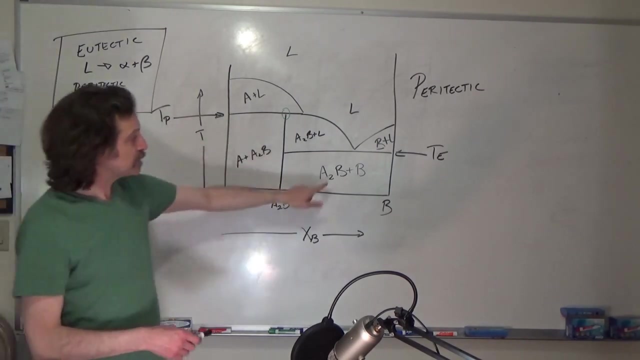 go back to the other side and work your way across, and typically That way you'll wind up with Meeting in the middle. In this diagram we've got a paratactic, which is happening there, and we have a eutectic, which is happening here. 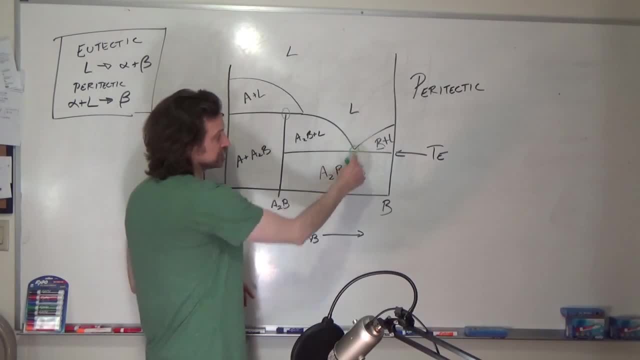 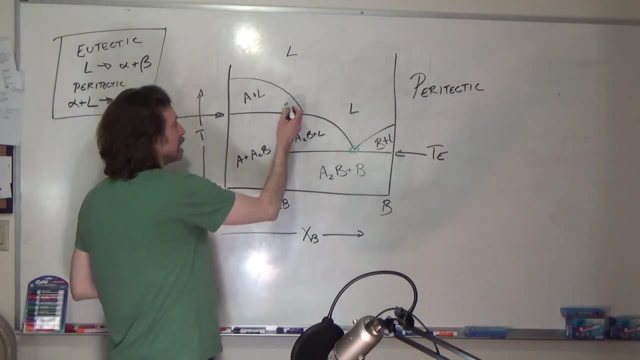 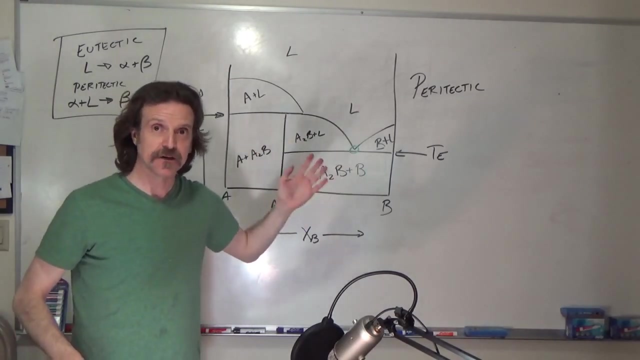 So again that eutectic Liquid turns into two solids and paratactic a, A plus L. Right, at that composition and at that temperature, transforms into Transforms, into a single phase. so that's what the paratactic is Now Reading. this is exactly the same as reading any binary phase diagram. right, your liquid, you cool down. 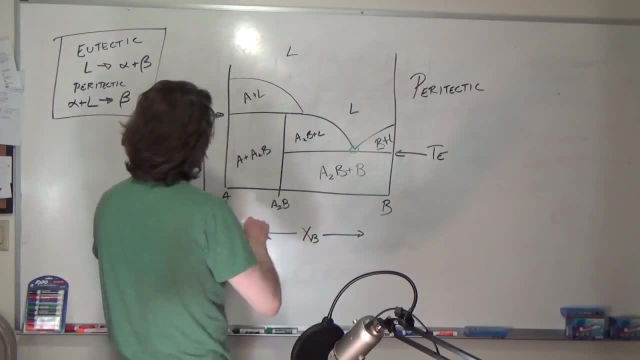 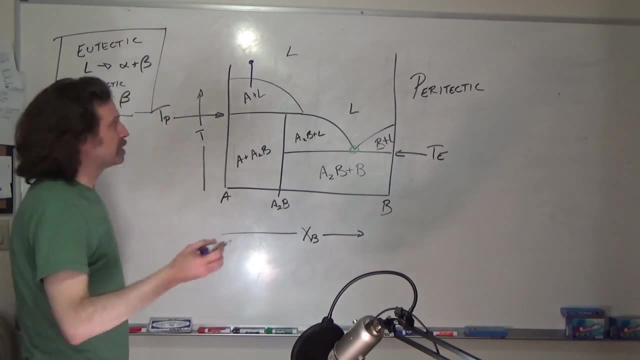 Let's. let's do an example here. Your liquid, you cool down. Going to a two-phase region say, okay, I'll draw my horizontal line. I got my tie line. I can read the composition of my solid, which is pure a. I can read the composition of my liquid. 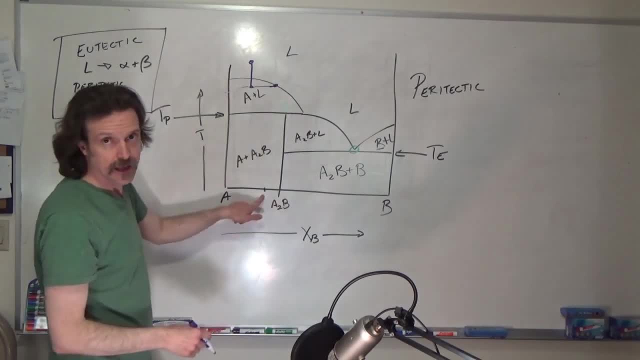 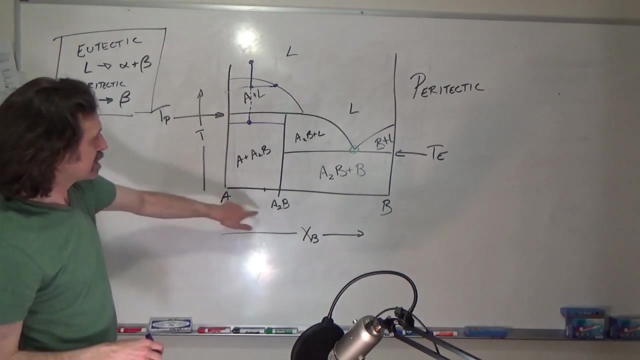 which read down here. I Can then use the inverse lever rule to figure out the phase fraction. right, simple, keep going down in this region. I've got you know a to be. I Can use the inverse level rule. This is all exactly as we've seen before. 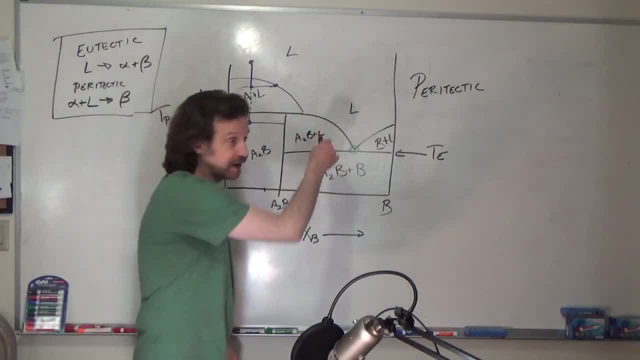 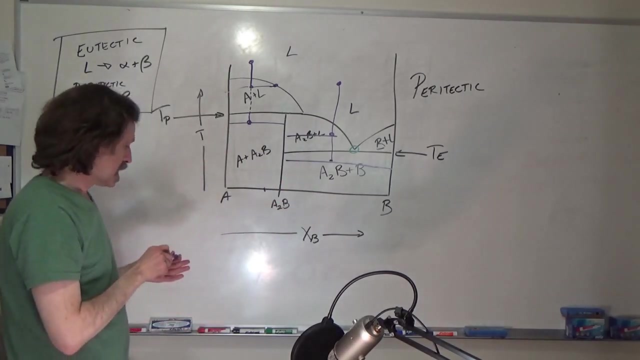 The thing that is. and over on this side I should point out: Yeah, the same thing as well. right, you say you're here cool down a to B plus liquid And here a to B plus B, right, no surprise, The thing that's surprising and what makes that. 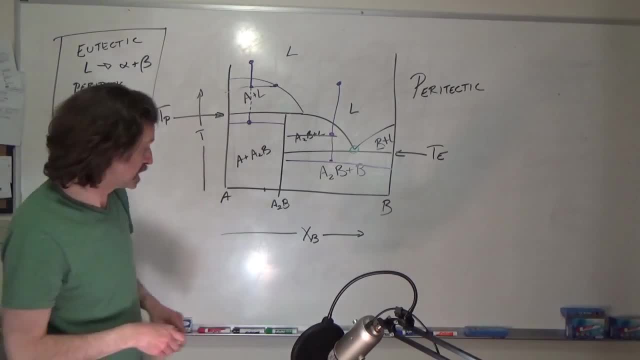 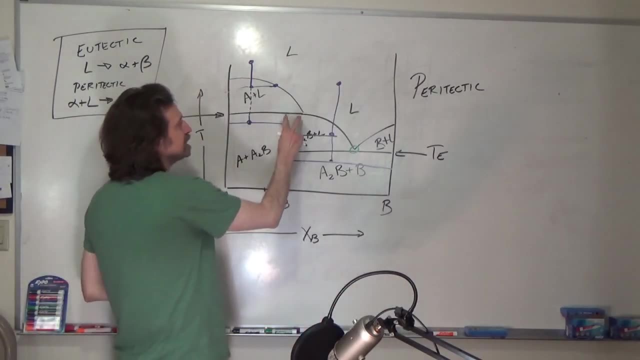 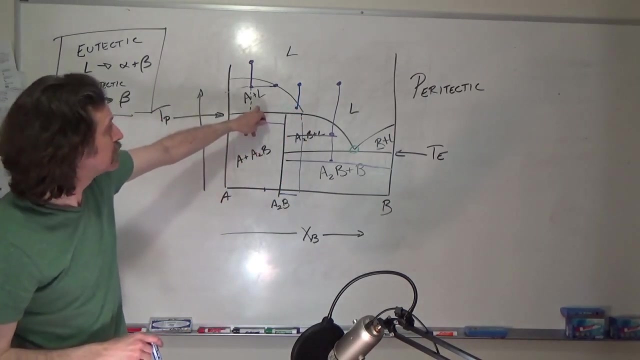 The paratactic. actually kind of- at least from my perspective, kind of interesting is that Between these two points, If you have a composition which sits Anywhere in here, as you cool down liquid, You form alpha plus liquid. Okay, You keep cooling down Right before you cross the paratactic temperature. 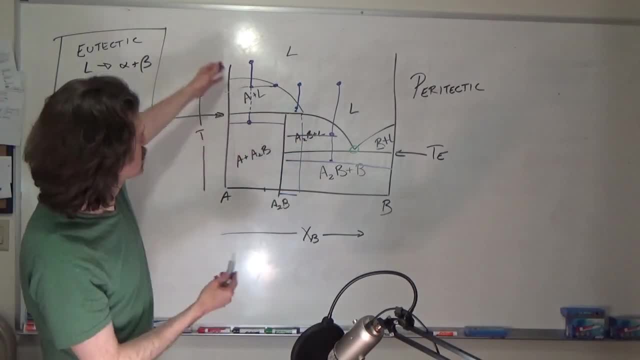 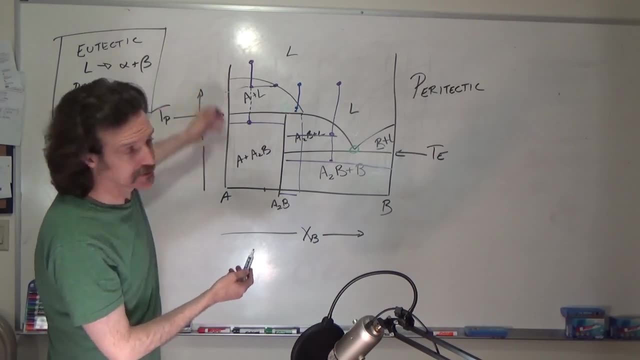 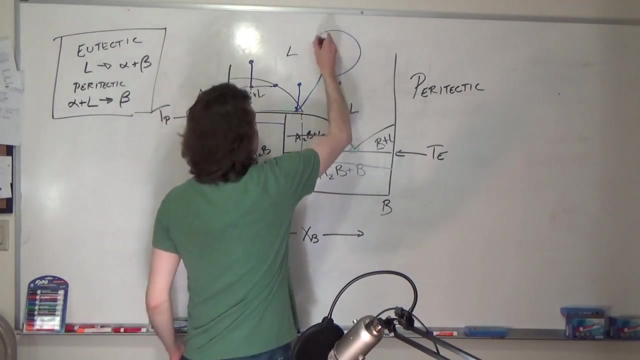 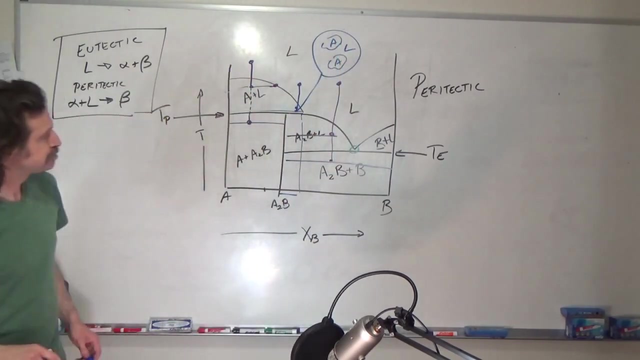 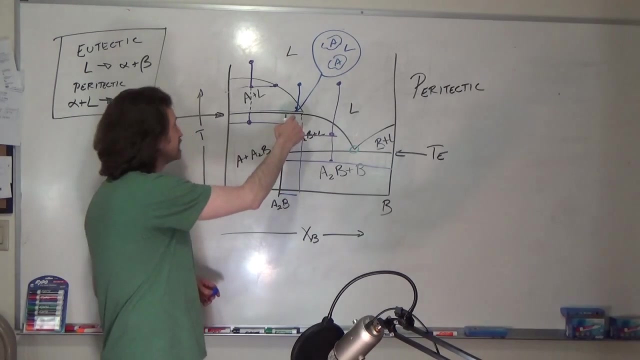 You can do your inverse level rule. you figure out. it looks like in this case It's going to be No, maybe 10% solid, right, so right here. And all the rest is liquid. Now what happens when you drop below the paratactic temperature? 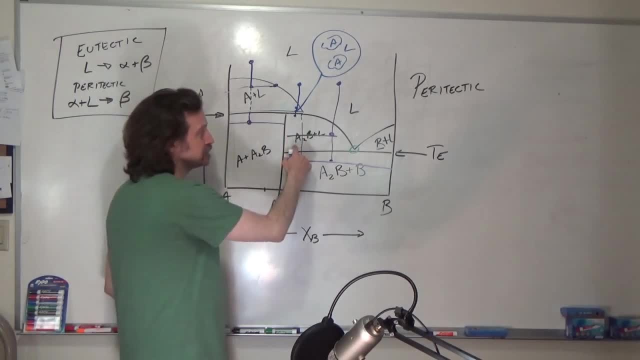 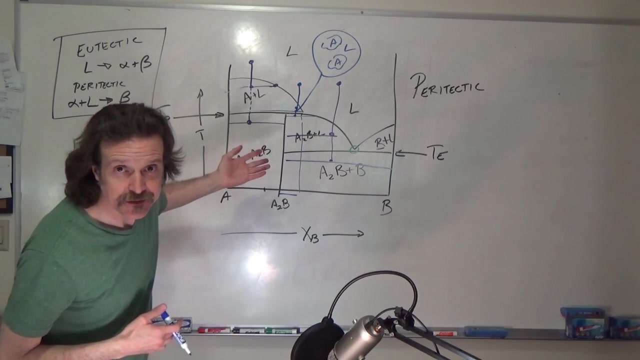 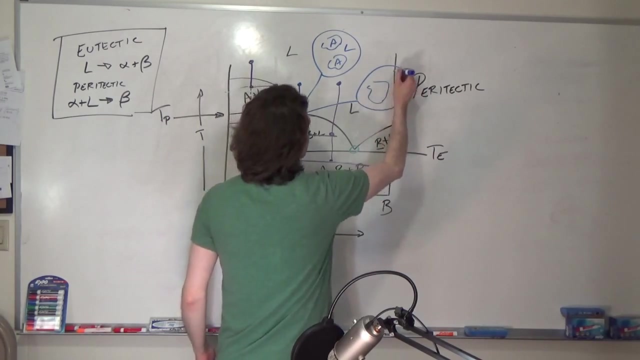 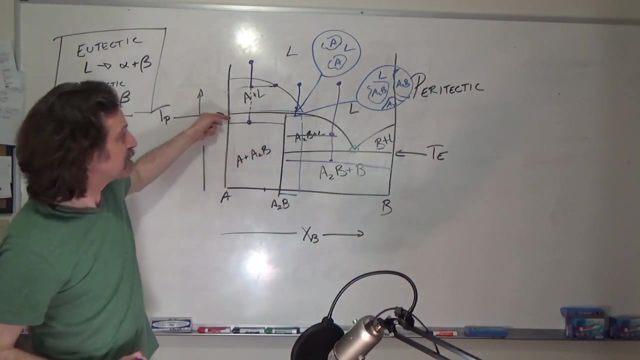 Well, now You're in a two-phase region which is a to B, plus liquid, and a to B. if I draw my horizontal tie line, It looks like it's maybe a two-thirds A to B, a to B, A to b. So in the process of changing temperature by, you know, one degree, 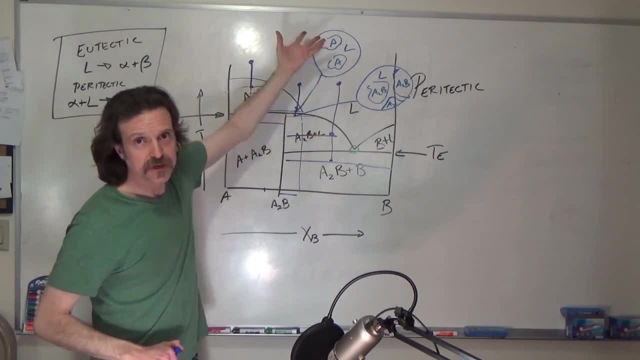 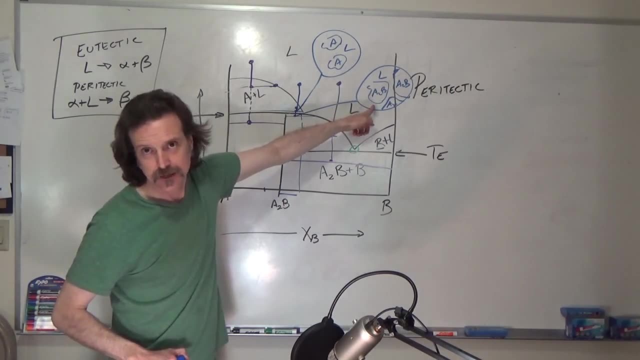 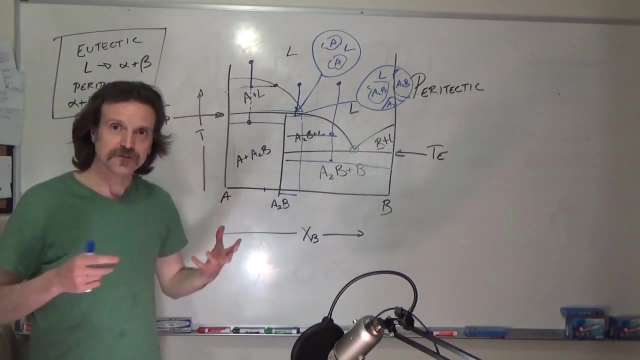 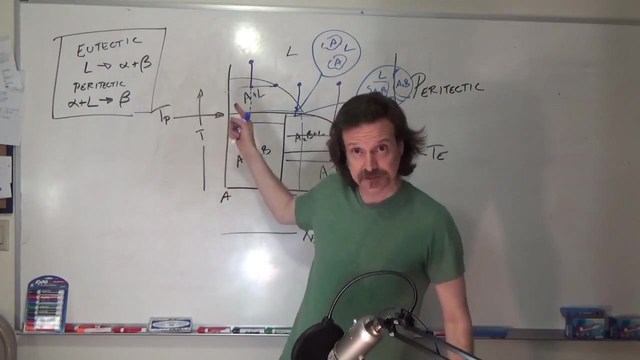 all of the A phase gets reabsorbed into liquid and a whole separate phase precipitates out. and that's what makes this kind of interesting, because you have all of this motion happening and as we go on and we talk about kinetic, some the kinetics of this is pretty. 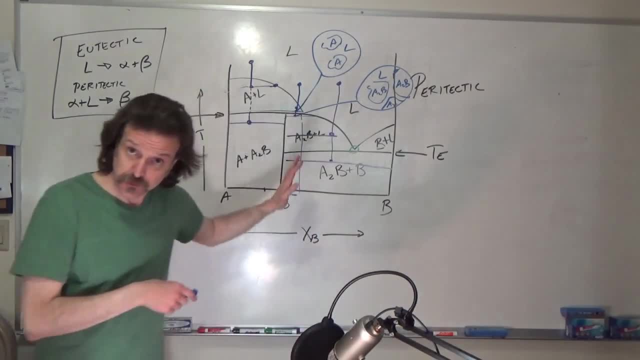 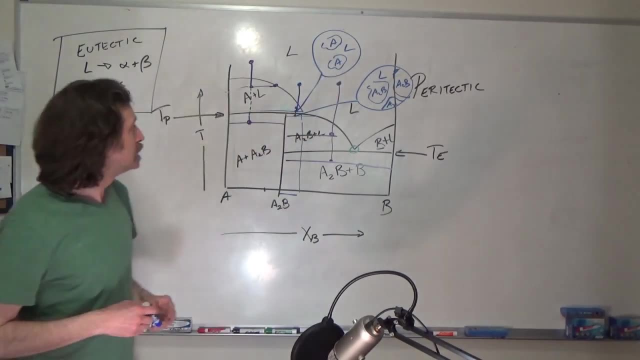 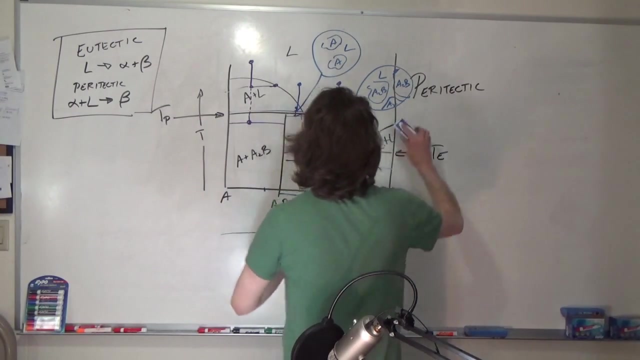 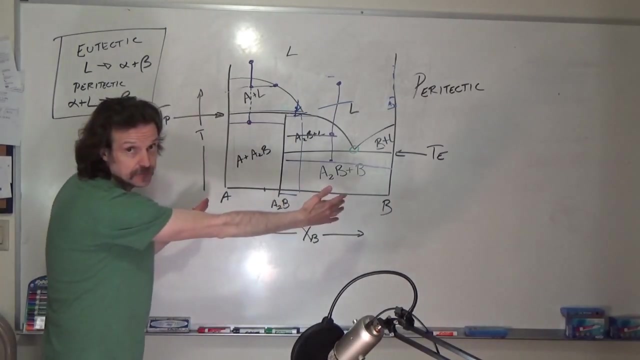 complicated and it gives us a lot of ways that we can control the microstructure, but you have this reabsorption event, so the way that you make sure you don't mess this up is simply through looking at the bottom of the phase diagram, and what I mean is that we know that we have these. 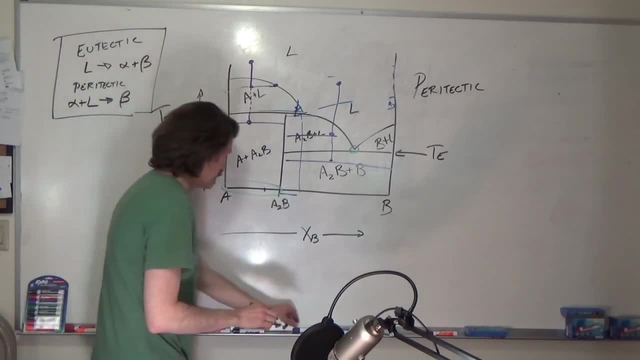 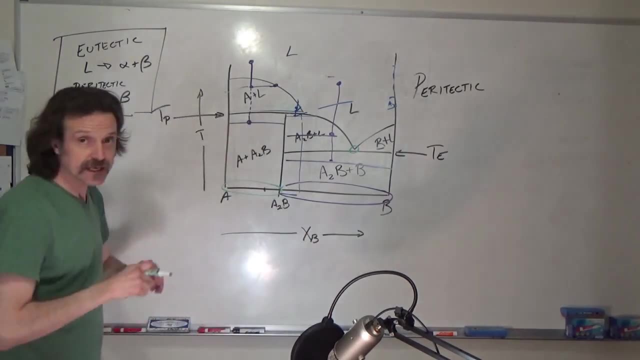 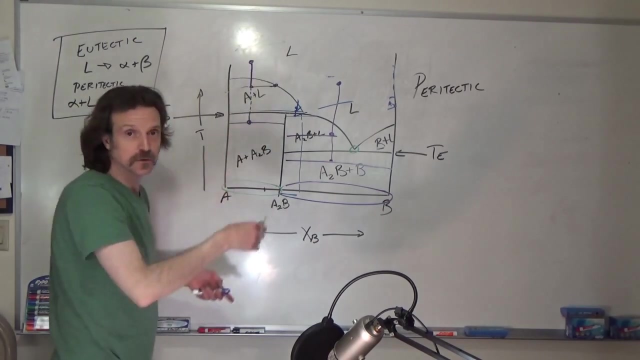 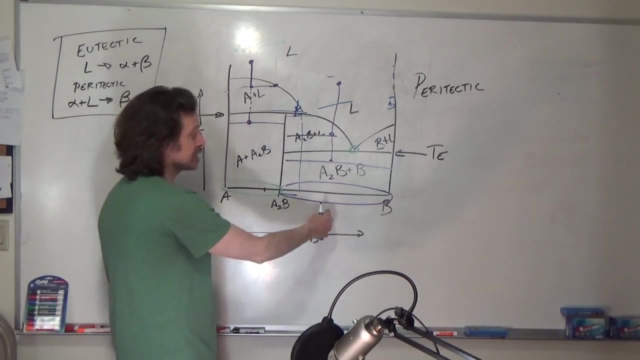 compositional regions here, and we have a compositional region here and we have a compositional region here. any system that sits between a and a to B up here, when it cools down it has to be made of the a and a to B phase a system that has. 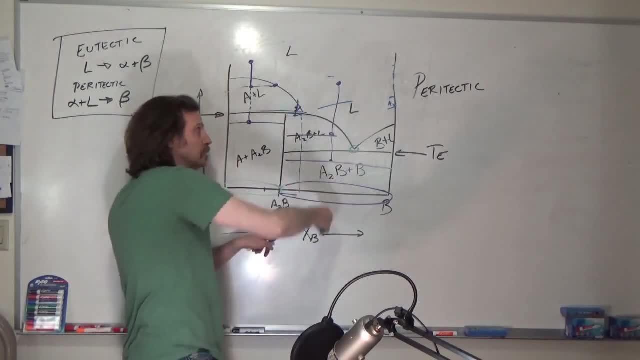 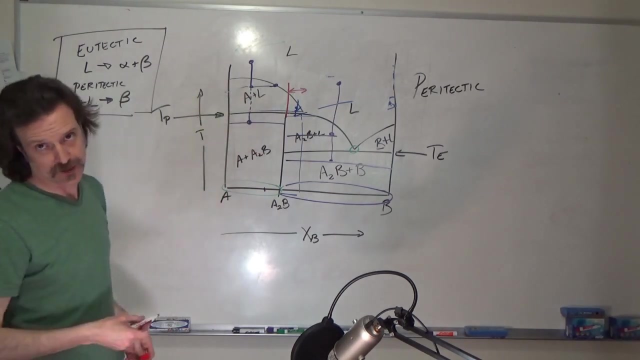 a composition between a to B and B. when it cools down it has to form a to B plus B, and the fact that we have this little weirdo region that starts out with a plus L that has to be transient as we cool down. it has to go away. so the way. 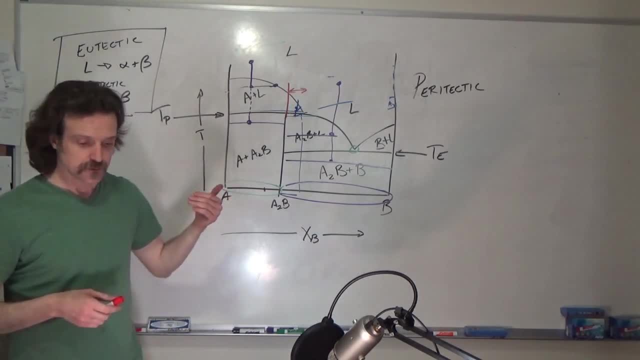 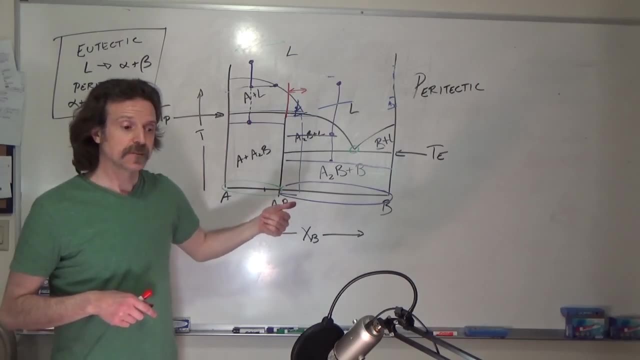 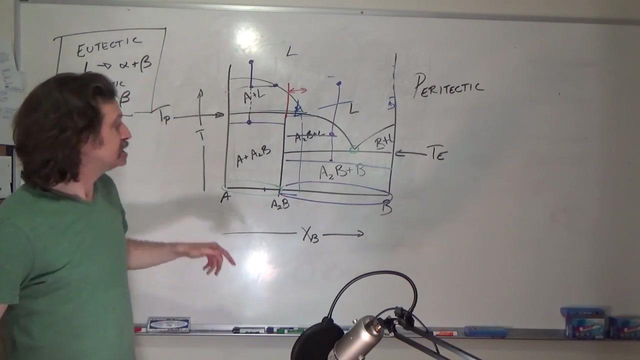 to make certain that you are properly identifying phases and that you properly identify the phase at that time. that's what I'm trying to do- the phases that actually form in your microstructure is to not only look at where you are in the phase diagram, but to always keep in mind the compositional ranges that your system 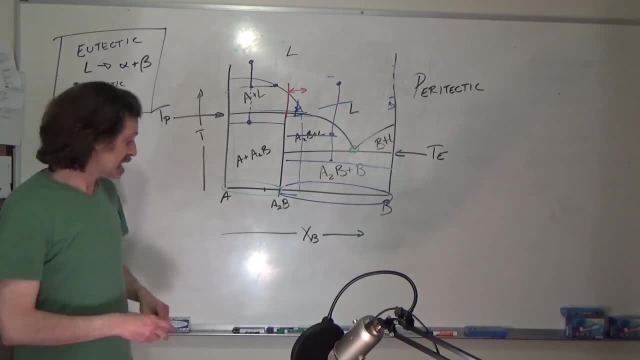 is sitting in And that will tell you where you have to end as you cool down and approach low temperature.